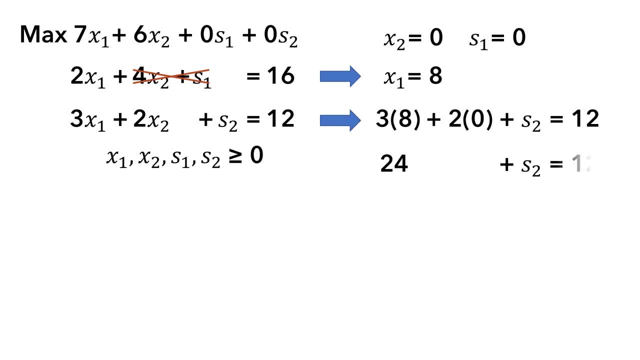 then X1 equals 8.. Plugging that into the second equation, we obtain S2 equals negative 12.. This is called a basic solution. However, it is not feasible because S2 equals negative 12 violates the non-negativity requirement. X2 and S1 that are set to zero here are called: 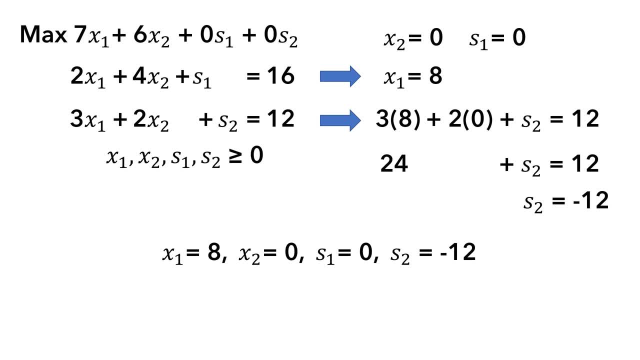 non-basic variables, while X1 and S2 are called basic variables. Usually we start by setting X1 and X2 to zero. In that case, S1 will be 16 and S2 will be 12.. In essence, we've made X1 and X2 non-basic, so that S1 and S2 are the basic variables. 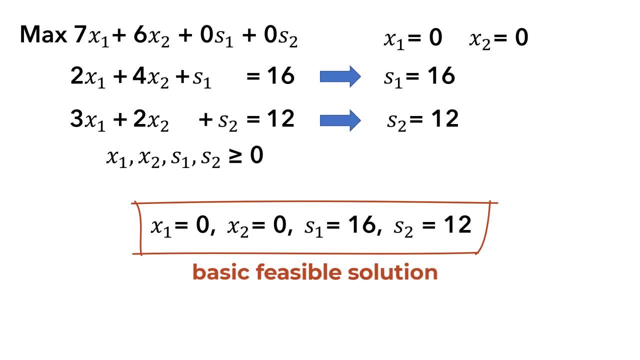 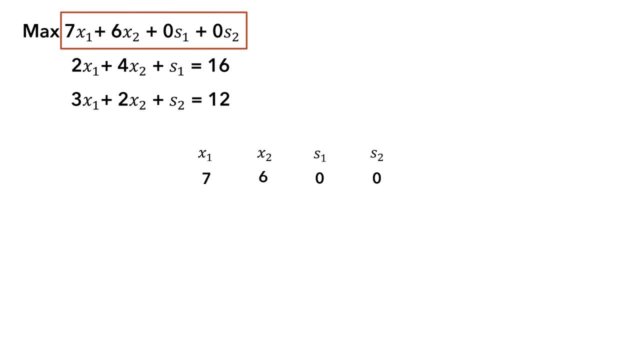 This is called a basic feasible solution. Feasible because it satisfies non-negativity as well. To set this up in a simplex tableau, we can begin with the objective coefficient row, which we call the C row or the Cj row, then the coefficients of the variables in the 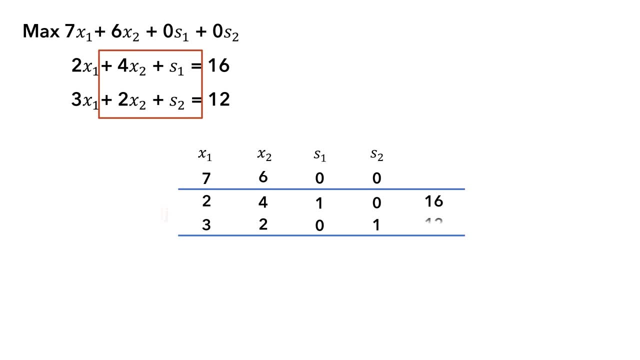 constraint, which we refer to as the A matrix, and their right sides called the B column or quantity column. Since S1 and S2 have one in their columns, with the other value being zero, they are called basic variables. These are also referred to as unit columns. 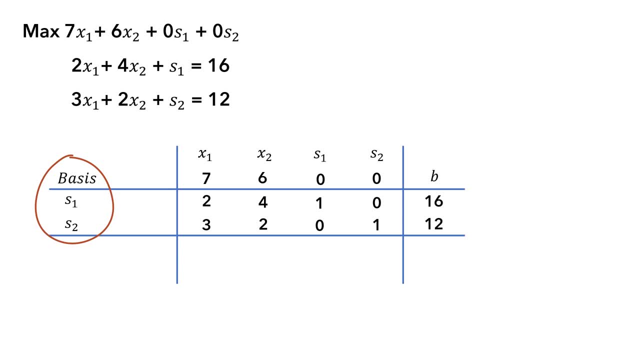 Next we place the basic variables in a column called basis here and place the objective function coefficients next to them in a column we refer to as the CB column. This shows that the initial basic feasible solution is S1 equals 16 and S2 equals 12.. Next we introduce the Zj row. 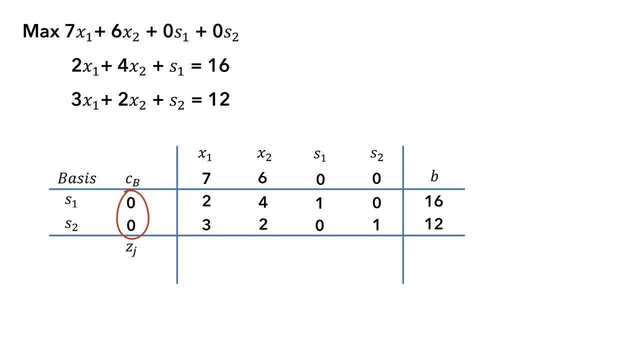 whose values are calculated by multiplying the CB values by the corresponding column values and adding the result. So for X1, it will be 0 times 2 plus 0 times 3,, which gives zero, And for X2, 0 times 4 plus 0 times 2,, which again is zero, And it will be zero for the rest as well. 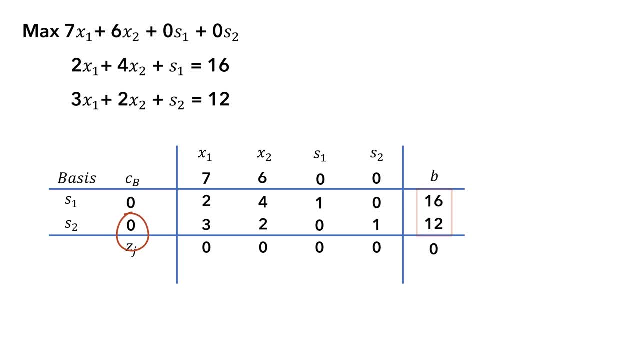 Our current objective function value will also be zero. here The Zj value for basic variables represent their unit contribution to the objective function value or profit, But for the non-basic variables it represents the amount of profit forgone or given up if a unit of the variable is added to the current solution. 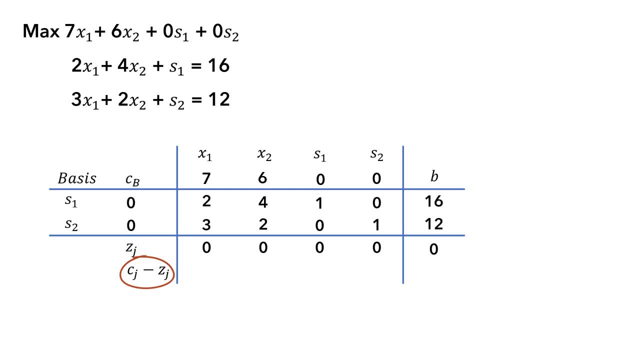 Next we have the Cj minus Zj row, which is calculated by taking each objective coefficient minus the Zj value. It represents the net change in the value of the objective function or profit, if one unit of each variable enters the solution. So it is referred to as the net. 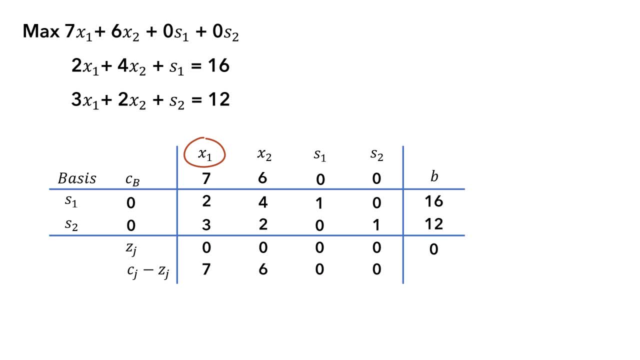 evaluation row. For example, if X1 enters the basis and its value increases by 1,, then the objective function increases by 7.. What we now have here is called the initial simplex tableau. It has a basic feasible solution: X1 and X2 equals 0,, S1 equals 16, and S2 equals 12.. X1 and X2 are equal to zero because they are. 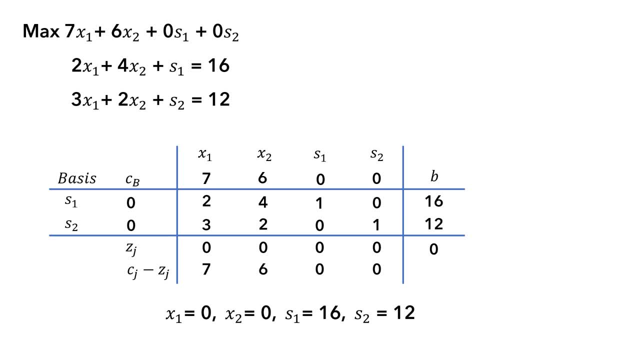 the non-basic variables. We now perform iterations until all values in the net evaluation row are either negative or zero. This happens when we reach an optimal solution. Next, to determine which of the non-basic variables to make basic, we select the entry with the highest positive value in the net evaluation row. That is the. 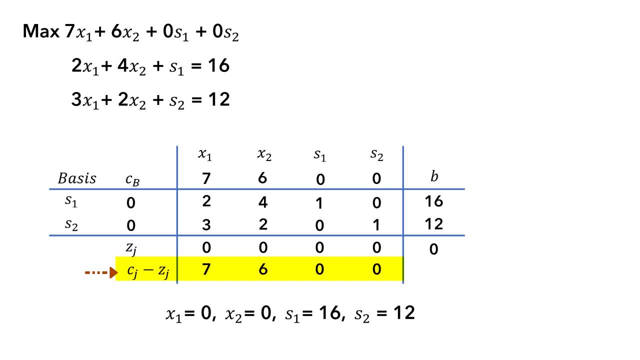 variable that provides the largest net improvement to the objective function. In this case the variable is X1, with the largest value of 7. here, If there is a tie, that is, if there is another 7 on this row, you can select any of them. but for consistency, 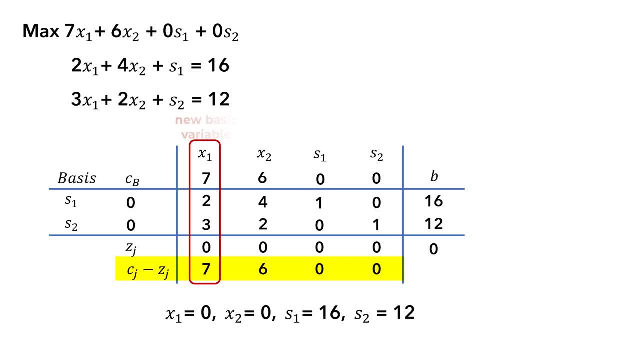 we prefer the leftmost one. So X1 would be the new basic variable. entering the basis, We refer to the corresponding column as the key column or pivot column. But which current basic variable will X1 replace S1 or S2? To determine that we calculate ratios of the B column values. 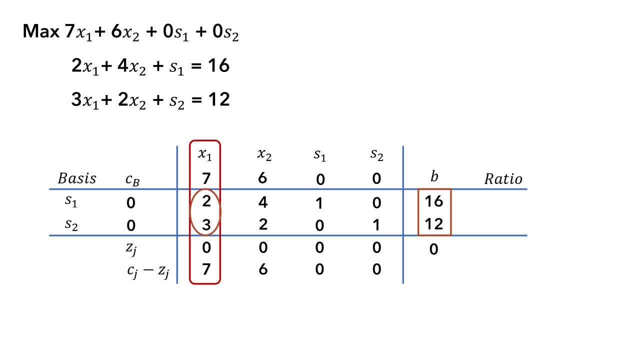 relative to their corresponding pivot column values and choose the row with the minimum value. For the first row, the ratio is 16 over 2, which gives 8.. And for the second row, the ratio is 12 over 3,, which gives 4.. The minimum of these two is 4.. Therefore, 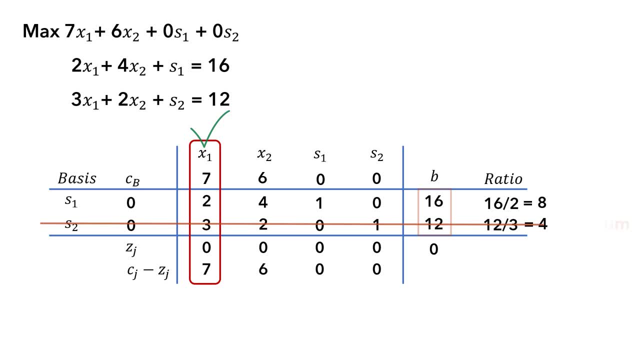 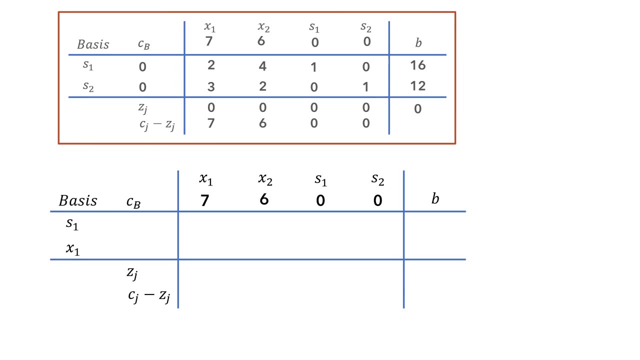 S2 will be leaving the basis. This row with the minimum value is called the key row or pivot row, and the value at the intersection of the pivot row and pivot column is referred to as the key element or pivot element. This again is the initial simplex tableau And 3 here is a pivot element. 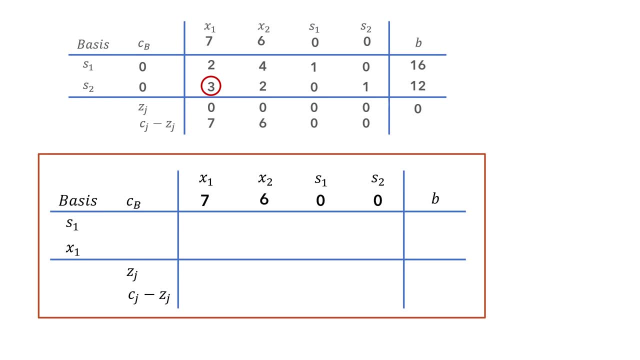 We will perform the first iteration down here. As noted earlier, S2 left the basis and has been replaced by X1, while S1 is still in the basis. The coefficient of S1 in the objective function is 0 and the coefficient of X1 is 7.. We now apply what we call elementary row. 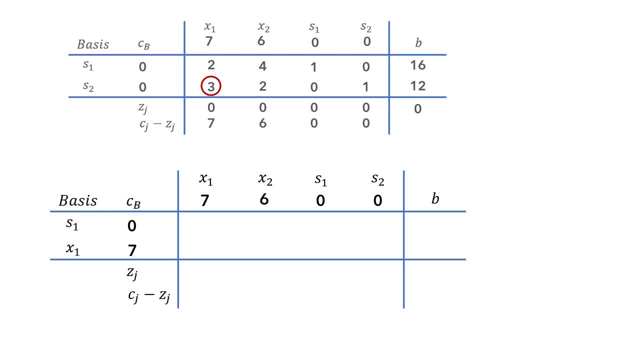 operations to manipulate the tableau element so that the pivot column becomes a unit column. In essence, we convert the pivot element to 1 and the other values in that column to 0.. To do that, we divide all the entries in the pivot row by the pivot element, which is 3.. 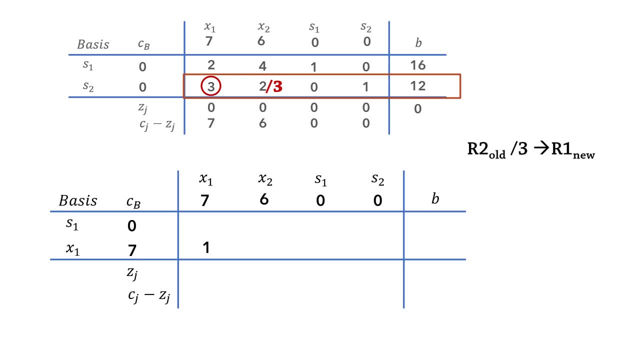 So 3 divided by 3 is 1.. 2 divided by 3 is 2 thirds, 0 over 3 is 0.. 1 over 3 is 1 thirds And 12 over 3 is 4.. Next we need to convert these two to 0,. 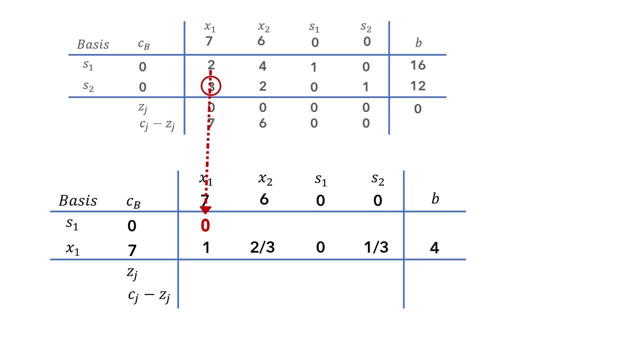 either by adding or subtracting a multiple of the unit pivot element from it. And whatever operation we perform to make these two a 0, we perform it on all other elements in that row. Now, to make these two a 0, we can multiply this 1 by 2. 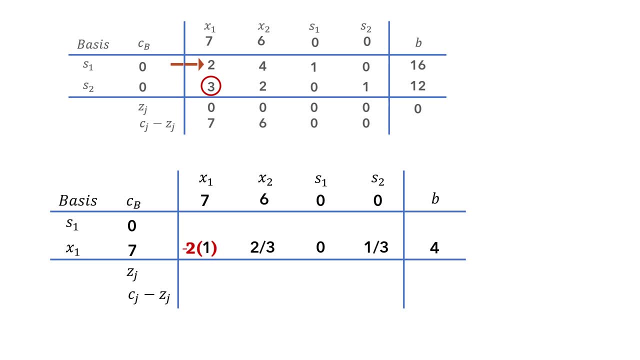 and subtract it from these two. In essence, the elementary row operation is this: We take a row 1 element subtract 2 times the corresponding new row 2 element and add a new row 2 element from that row. We take a row 1 element subtract 2 times the 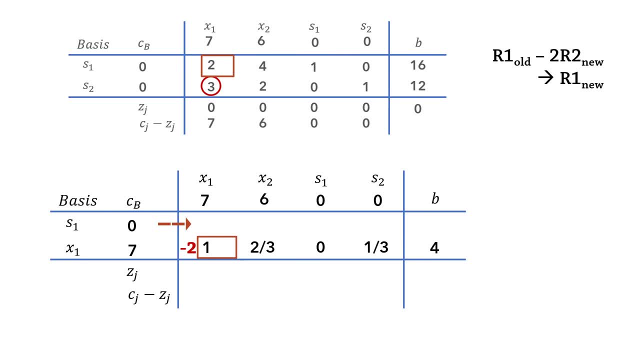 corresponding new row 2 element and assign the result to the new row 1 element. So 2 minus 2 times 1 is 0, as advertised. 4 minus 2 times 2 thirds is 8 thirds. 1 minus 2 times 0 is 1.. 0 minus 2, 1 third is negative 2 thirds. 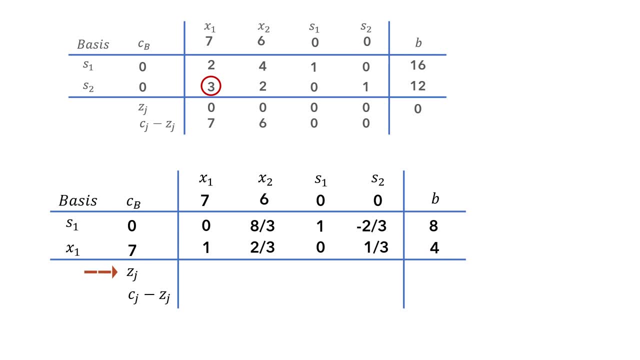 And 16 minus 2 times 4 is 8.. For Zj we take the sum of the products, of the objective coefficients, of the basic variables and the columns. So for the first column we have 0 times 0 plus 7 times 1, which gives 7.. 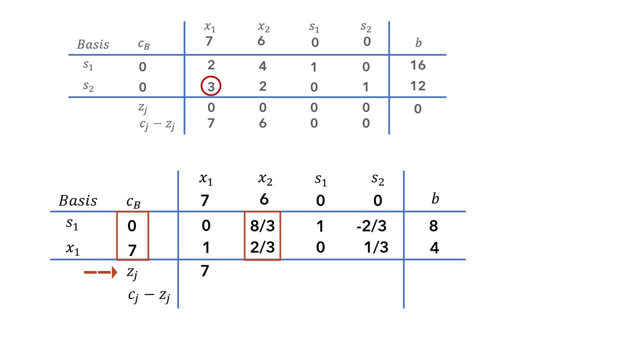 For X2 column, we have 0 times 8 thirds plus 7 times 2 thirds, which gives 14 thirds. 0 times 1 plus 7 times 0 gives 0. This one gives 7 thirds. And for the B column we have 0 times 8 plus 7 times 4, which gives 28.. 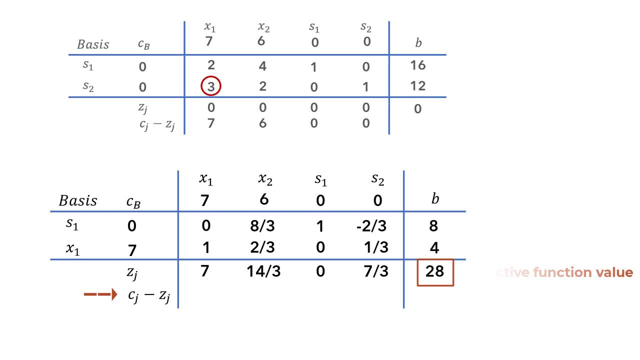 And that is the profit for the current solution. For the net evaluation row, we compute coefficients minus Zj values. 7 minus 7 gives 0.. 6 minus 14 thirds gives 4 thirds. 0 minus 0 gives 0.. 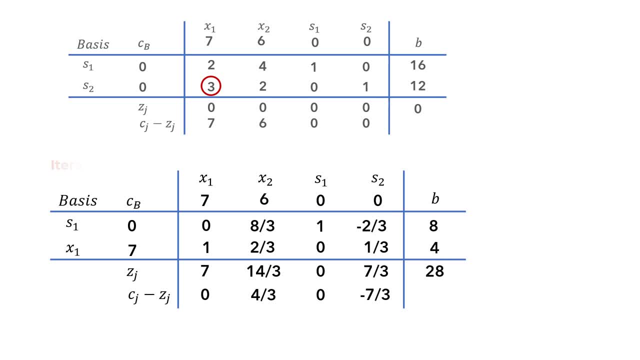 0 minus 7 thirds gives negative 7 thirds. The first iteration is now done. We have a feasible solution of S1 equals 8,, X1 equals 4, and the objective function value is 28.. This is, however, not optimal yet, since we still have a positive value in the net evaluation row. 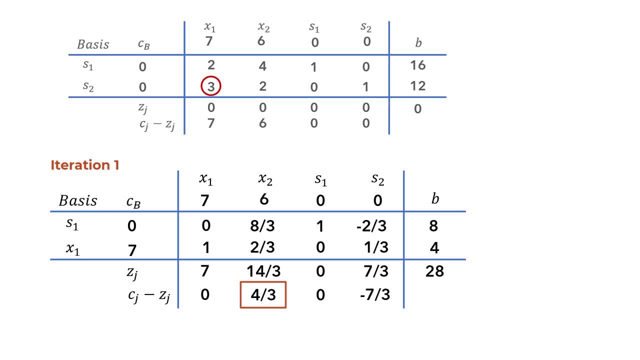 indicating that the profit can still improve. Recall that for our optimal solution, each Cj minus Zj must be less or equal to 0. Hence we move on to our next iteration. The new pivot column again will be the one with the most positive net evaluation entry. 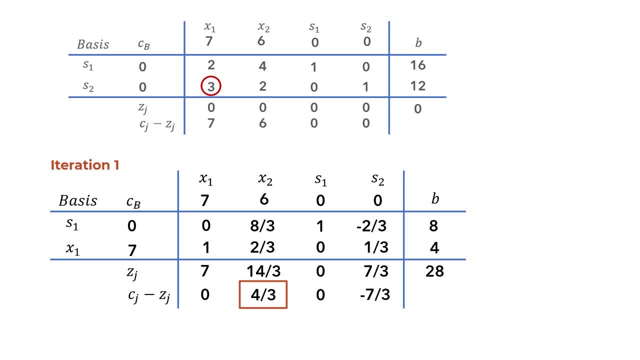 that is the variable that will bring the greatest improvement to the objective function value, which is X2 in this case. To determine the pivot row, we divide the B column values by the positive pivot column values and select the row with the minimum ratio. 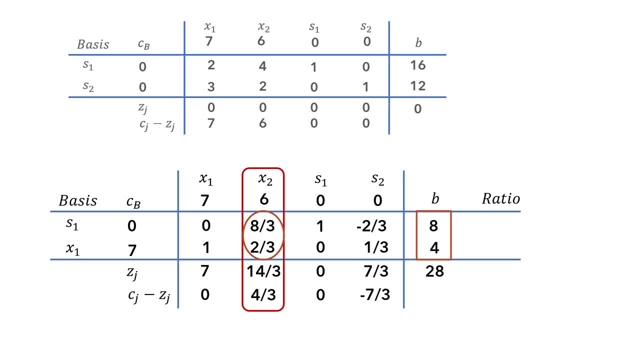 So 8 divided by 8 thirds is 8 times 3 over 8, which gives 3.. And 4 divided by 2 thirds is 4 times 3 over 2, which gives 6.. The minimum of the two ratios is 3.. Therefore, the S1 row is the pivot row. 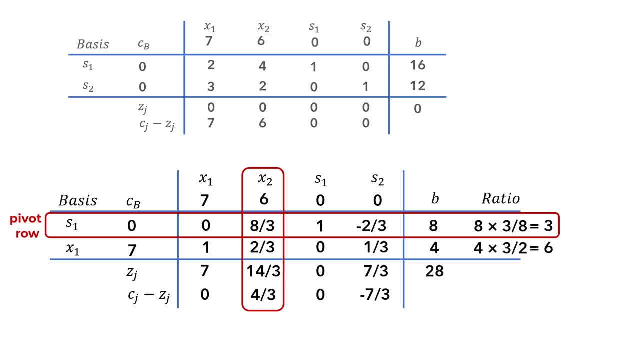 If there is a tie in the ratios, that is suppose this 6 is also a 3, we can choose any of the two, but we will prefer to choose the topmost one for consistency. Now recall that the basic variable in the pivot row will be leaving the basis. 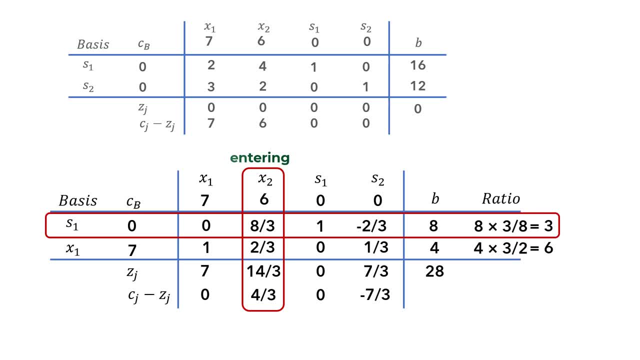 and the non-basic variable in the pivot column will be entering it. In essence, S1 will be leaving the basis and X2 will be replacing it, And 8 over 3 is the key or pivot element, as it is at the intersection of the pivot row and pivot column. 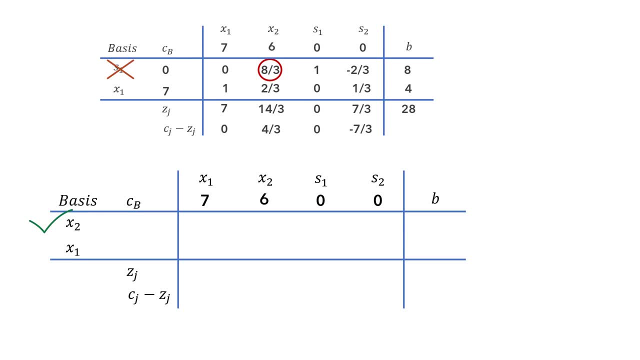 For the next iteration. X2 replaces S1 here and will place its objective function, coefficient 6, in the CB column. here X1 stays with its coefficient of 7.. Next we convert the pivot element to 1 in the new tableau by dividing the entries in: 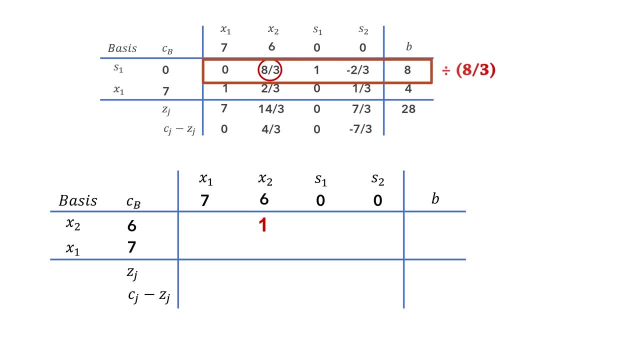 the current pivot column by 8 thirds, That is, multiplying them by 3 over 8.. So 3 over 8 times 0 is 0.. 3 over 8 times 8 thirds is 1, as expected. 3 over 8 times 1 is 3 over 8.. 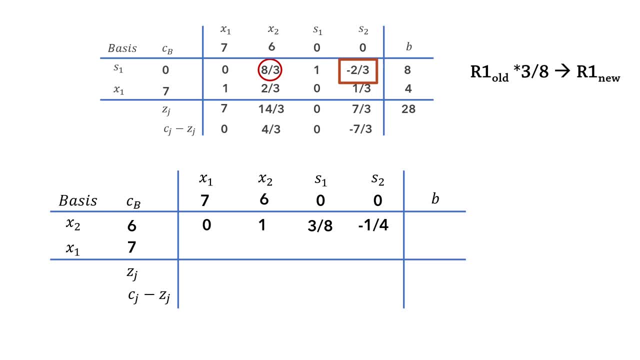 3 over 8 times negative. 2 thirds is negative 1 quarter, And 3 over 8 times 8 is 3.. Next we make this column a unit column by making this entry in row 2: 0.. To do that, we multiply this new row 1 by 2 thirds and then subtract it from the current row 2.. 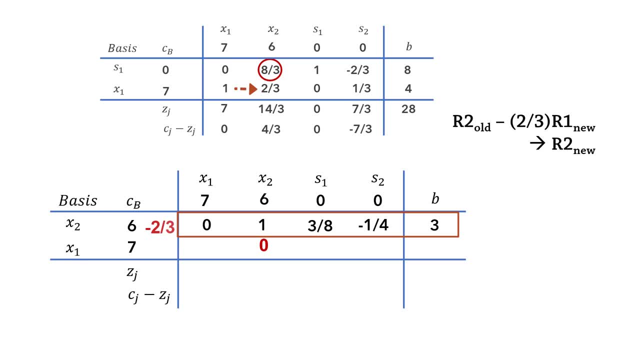 That is old row 2 values minus 2 thirds times new row 1 values will be assigned to the new row 2.. So 2 thirds minus 2 thirds times 1 equals 0, as required For X1 column. 1 minus 2 thirds times 0 is 1.. 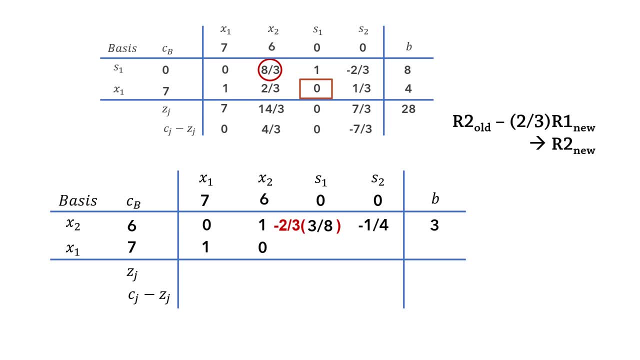 For S1 column: 0 minus 2 thirds times 3 over 8 is negative 1 quarter. 1 over 3 minus 2 thirds times negative. 1 over 4 is half. And for the B column, 4 minus 2 thirds times 3 equals 2.. 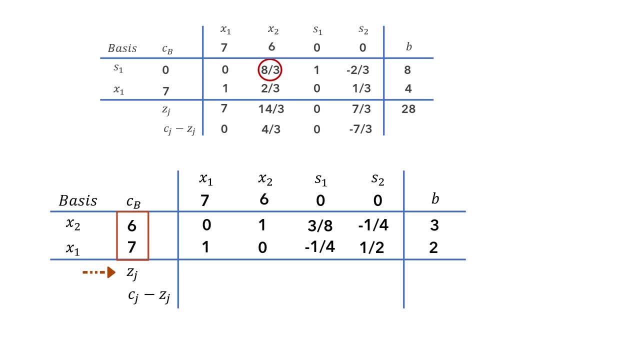 Next we calculate each Cj value by multiplying the basic objective coefficients by the column entries and adding the results. So 6 times 0 plus 7 times 1 equals 7.. 6 times 1 plus 7 times 0 equals 6.. 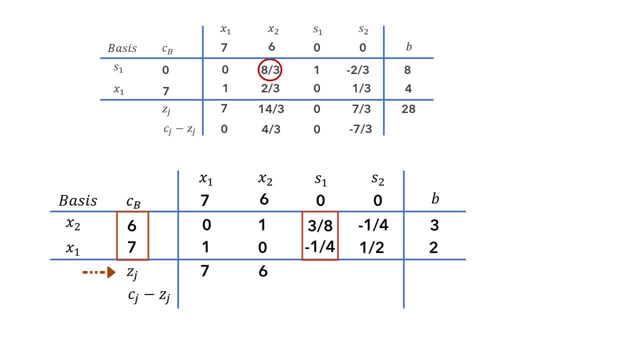 6 times 3 over 8 plus 7 times negative, 1 quarter equals half 6 times negative. a quarter plus 7 times half equals 2.. And for the B column, 6 times 3 plus 7 times 2 equals 32.. 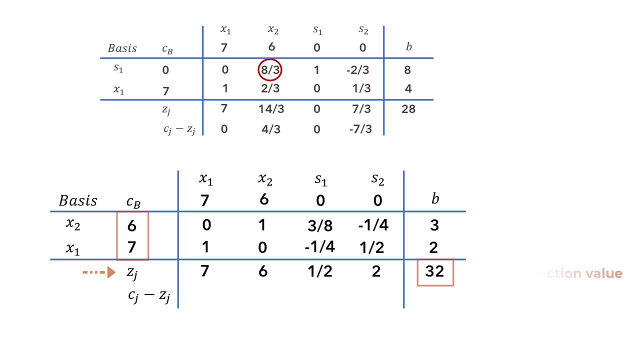 And that's the objective function value for this iteration. For the net evaluation row, we do 7 minus 7, which gives 0.. 6 minus 6 also gives 0.. And that's the objective function value for this iteration. So 0 minus half gives negative half. 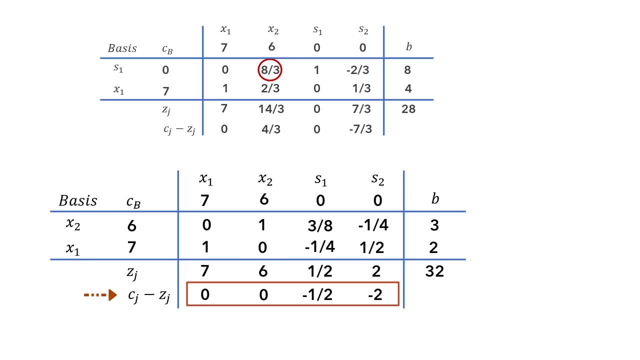 And 0 minus 2 gives negative 2.. Since all Cj minus Zj elements are non-positive, we can't improve on this solution. So this is our optimal solution: X1 equals 2.. X2 equals 3.. S1 and S2 will be zeros because they are non-basic. 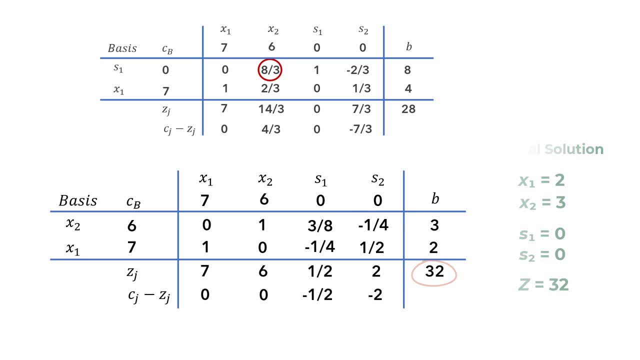 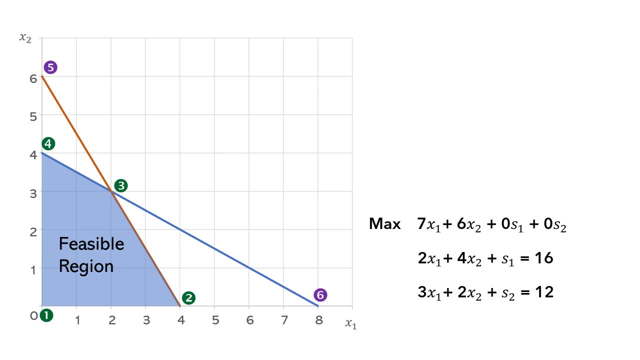 And the objective function value will be 32.. Now let's see how this relates to the graphical solution of the LP problem. The basic solutions are the extreme points labeled 1,, 2, 6.. The basic feasible solutions are the extreme or corner points of the feasible region, labeled 1,.